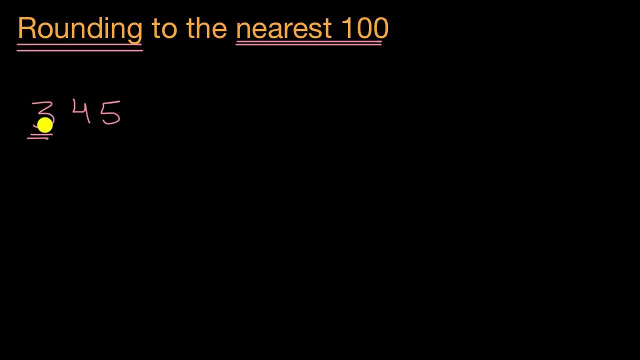 And what we want to do is first look at the hundreds place And you could see 345 is 300, 400's, four 10's and five ones, So 345, the 100, the number of 100's that is right below 345, is 300's. 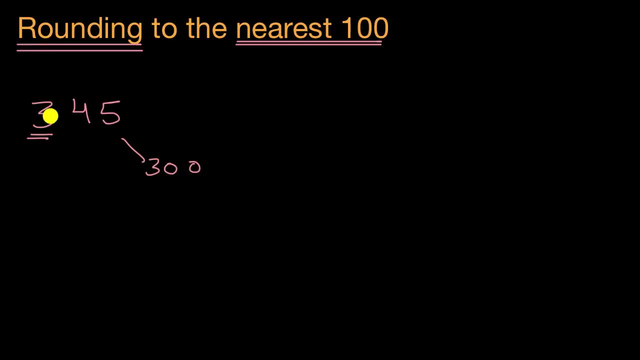 So it's between 300's, zero 10's and zero one's, And then the number of 100's, that's right above this number, is 400.. We're in between 300's and 400's And 400.. 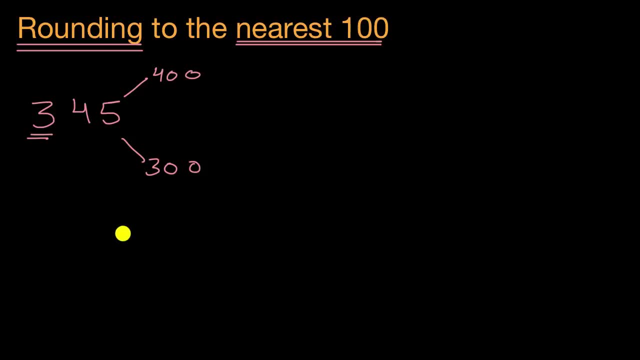 So if we're going to round this to the nearest 100, it's going to go to one of the hundreds: Three, four, 100, zero 10's and zero ones. these two, Well, to think about which one we round to. 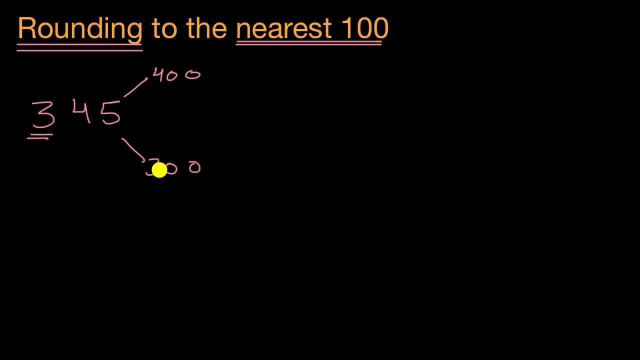 we have to think about: well, is 345 closer to 400, or is it closer to 300?? And to think about that we can draw ourselves a number line, And so let me just start my number line here at- I'll just start it at 200, so that's 200.. 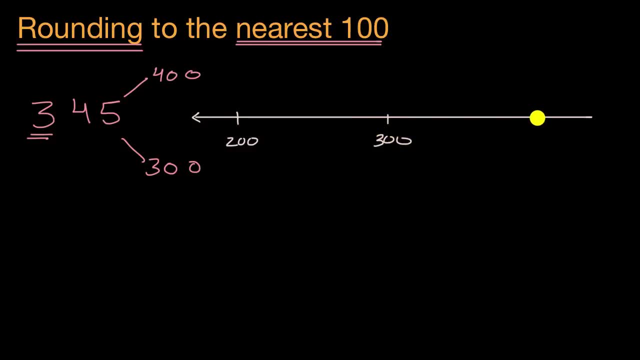 Let's make this 300. And then this would be 400. And then, since we let's just see this would be about 350 right over here, so I'll do the 50s right over there. so that's 350.. 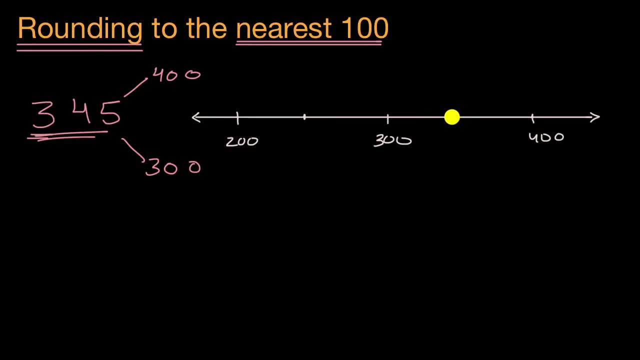 So where would 345 sit? Well, 345 is a little bit less than 350.. It's going to be roughly right over there. So which 100 is it closer to? Are we closer to 300, or are we closer to 400?? 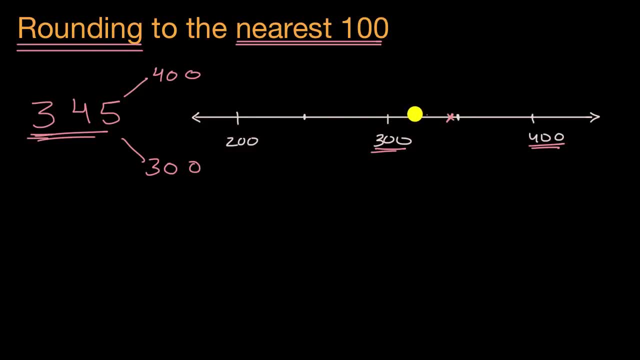 Well, you can visually see, 350 is right in between. It's 50 away from 300 and 50 away from 300. It's 50 away from 400.. So 345 is going to be a little bit closer to 300.. 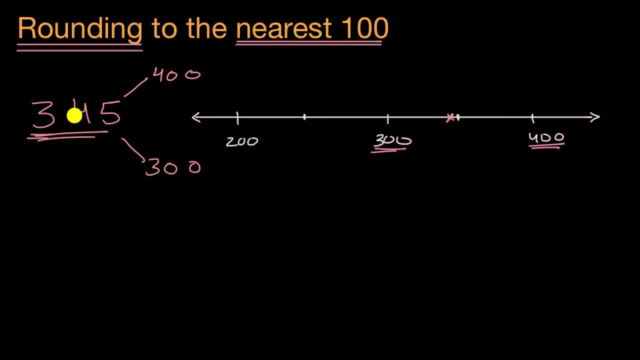 So in this situation, if we're rounding to the nearest 100, we would round down to 300.. Now, another way that you could do this- and it's very similar to what we thought about when we rounded to the nearest 10- is 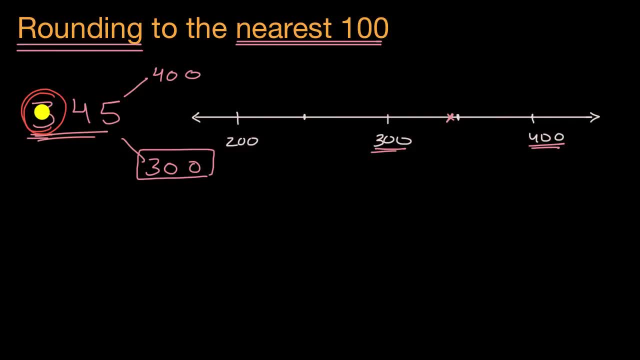 okay, we're rounding to the nearest 100.. So this is either going to be rounded to a three or a four And, to decide on that, we go to 1.5.. And, to decide on that, we would go to the 10s place. 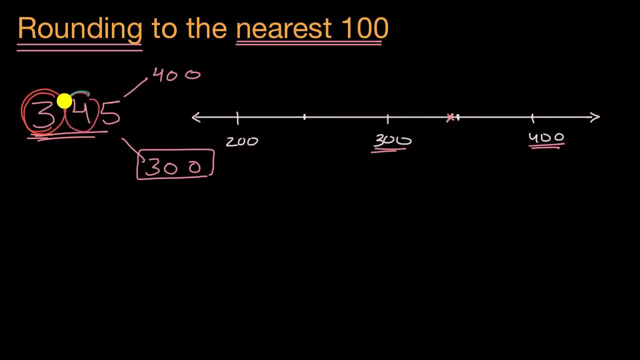 We do this in a different color. Go to the 10s place And in our 10s place right over here. if this is less than five, then we round down. If it is greater than or equal to five, we round up. 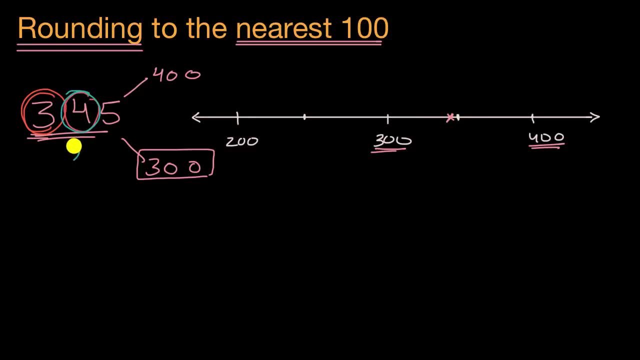 So in this situation, it is less than five. so we round down: If this was 365, well then that would be greater than or equal to five. So we round down. So in this situation, if this is less than or equal to five, 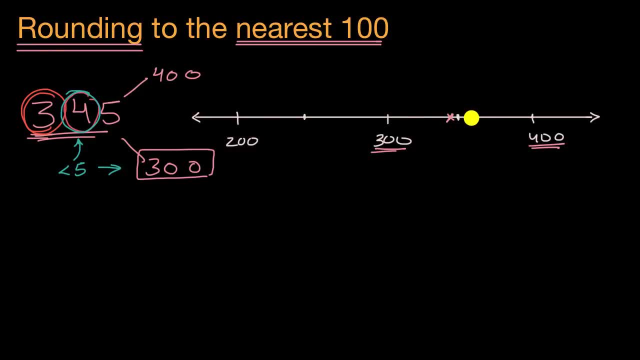 so then we would round up, And that makes sense, because 365 would be over here and it would be closer to 400.. Let's do another example. We'll do it both with what I just described and we'll do it with a number line. 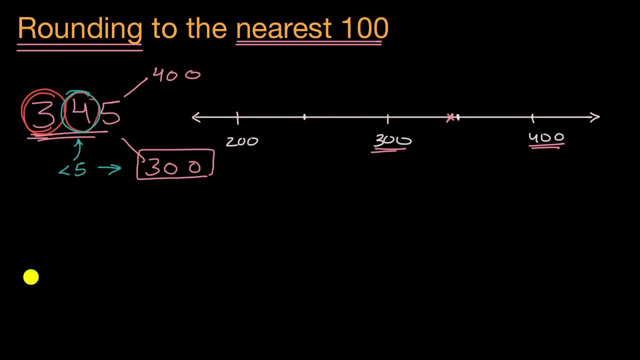 And I'll actually do a four-digit number now just to mix things up a little bit. Let's say we have the number 7,652.. Pause this video and see if you can round this number to the nearest 100.. All right, now let's do it together. 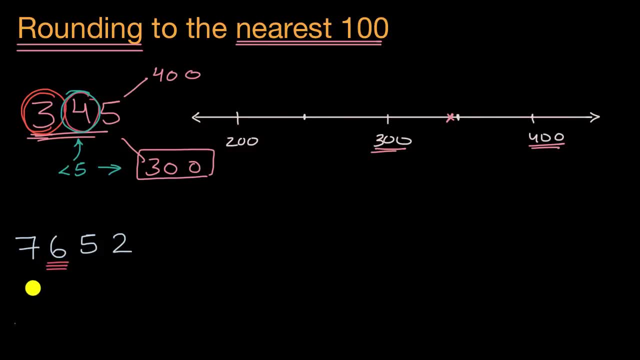 Now we're thinking about the hundreds place. So, right over there, you could view this as 7,600s, or you could even view this as 7,600s. So what are the closest hundreds to this number? Well, this is. you could either view this as 7,600s. 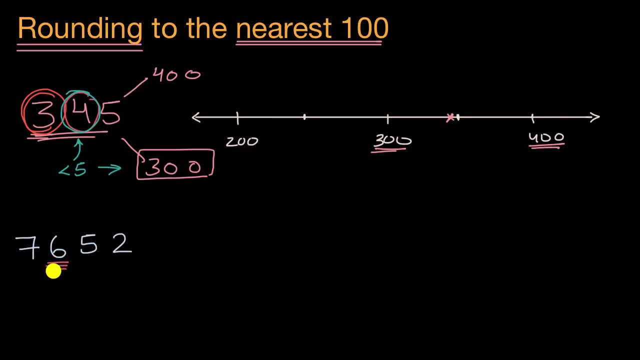 and five 10s and two ones, or 7,600s, five 10s and two ones, And so, either way, the hundreds that are right below this is 7,600s or 7,600.. And the hundreds that are right above this. 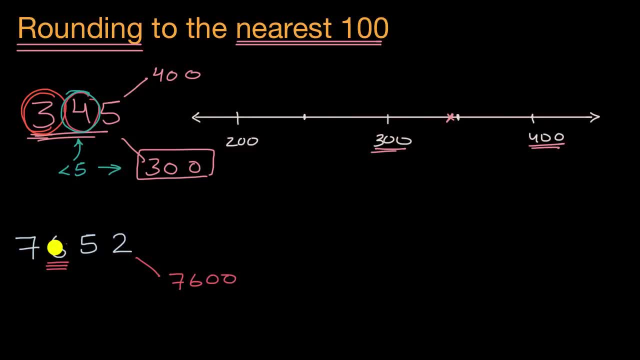 well, you would just take one more than this six, So that would be 7,700.. 7,700. And so which one would it round to? Well, we could use the technique that I just showed you. You go one place value less than the hundreds. 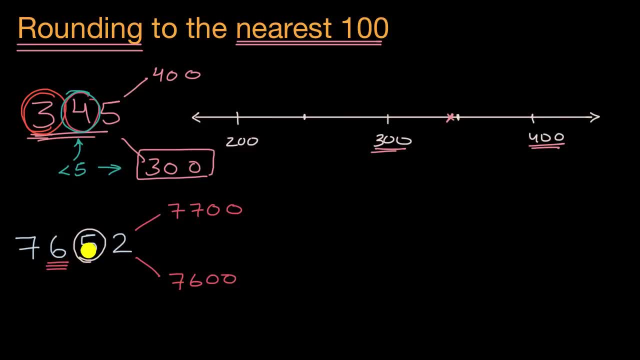 which, in this case, is in the 10s position, And you'd say: all right, is this greater than or equal to five? If it is, we round up. Is this less than five? Then we round down: This is greater than or equal to five.